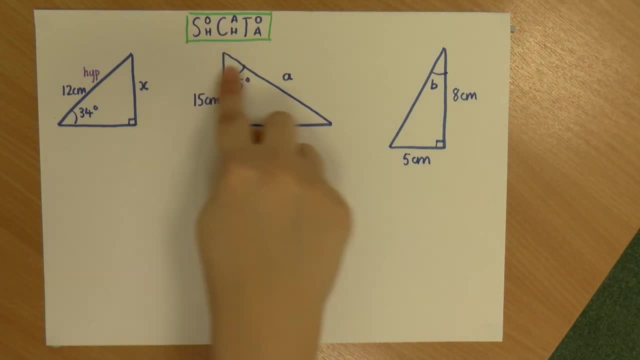 So, before we start answering any of these, we should be familiar with our acronym or equation for trigonometry. So it may be something that looks like this: SOHCAHTOA, or it may be something in a longer format, So I'm going to do one of each. so we'll talk about the. 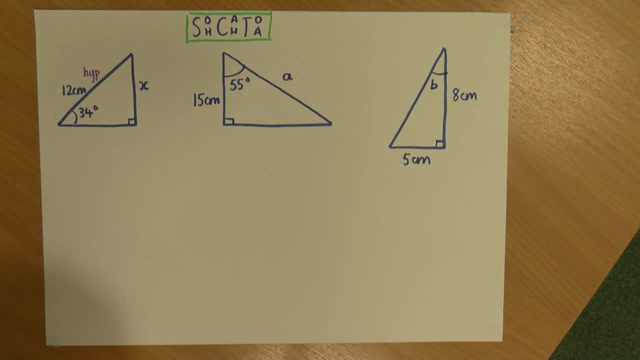 longer format as they come up, in case you recognise those easier. So let's start with hypotenuse, my opposite and my adjacent. Now the hypotenuse has already been identified. It is the longest side. it's the diagonal opposite, the right angle I now need to identify. 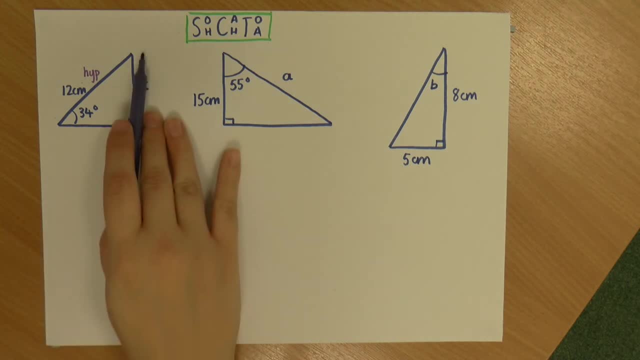 what my other two sides are. So on the right I've got my side x that is opposite the angle. so that is my opposite side, And if you're not comfortable with doing this, please do see my previous video on identifying the hypotenuse. 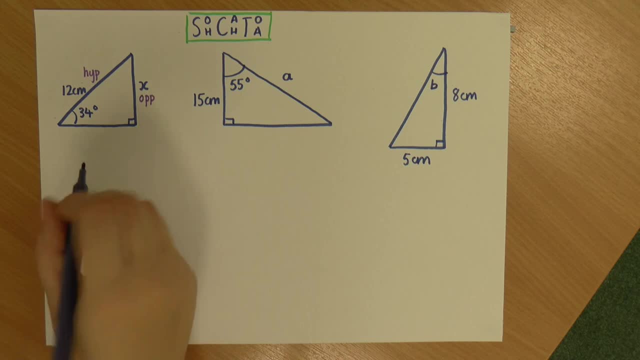 Subtitles by the Amaraorg community. opposite and adjacent, and that means that this side is the adjacent. So I have been given my hypotenuse and I have been asked to find my opposite, this side x. Okay, so using the hypotenuse and opposite, I can consult my equation, or: 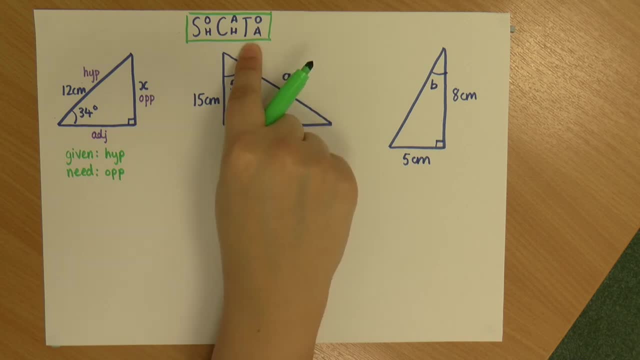 my acronym to find out which of these I have to use. So I'm using the hypotenuse H and opposite O, so it's the sign one I have to use. So it's that Now some of you may be more familiar with it. looking like. 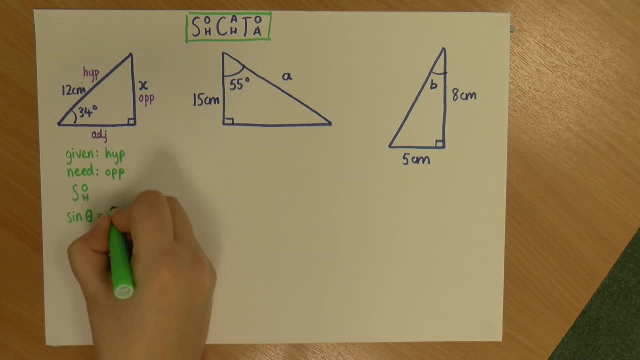 this, Something like that, probably with opposite and hypotenuse written out fully. I'm extremely lazy so I'm not going to write those out fully. but opposite is op, hypotenuse is hip And this symbol here is a theta. it may also say x instead of theta for angle. Okay so 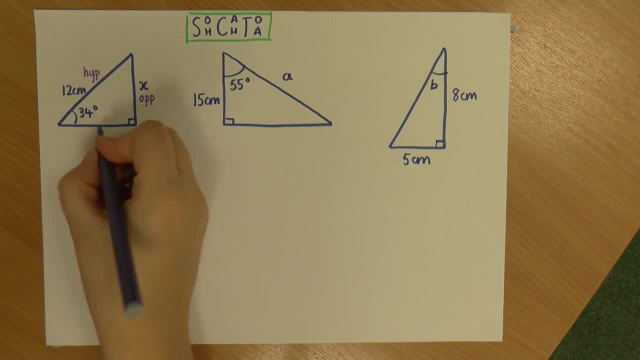 opposite and adjacent, and that means that this side is the adjacent. So I have been given my hypotenuse and I have been asked to find my opposite. this side x. Okay, so using the hypotenuse and opposite, I can consult my equation, or: 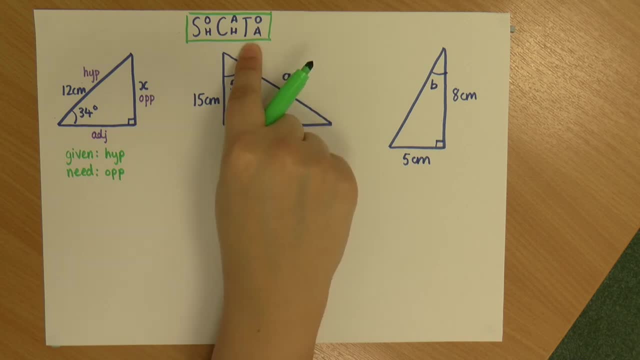 my acronym to find out which of these I have to use. So I'm using the hypotenuse H and opposite O, so it's the sign one I have to use. So it's that Now some of you may be more familiar with it. looking like. 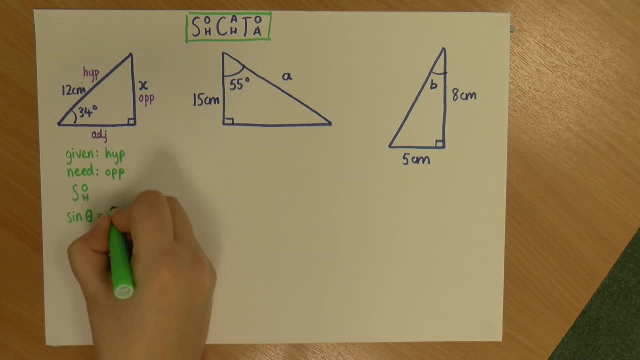 this, Something like that, probably with opposite and hypotenuse written out fully. I'm extremely lazy so I'm not going to write those out fully. but opposite is op, hypotenuse is hip And this symbol here is a theta. it may also say x instead of theta for angle. Okay so 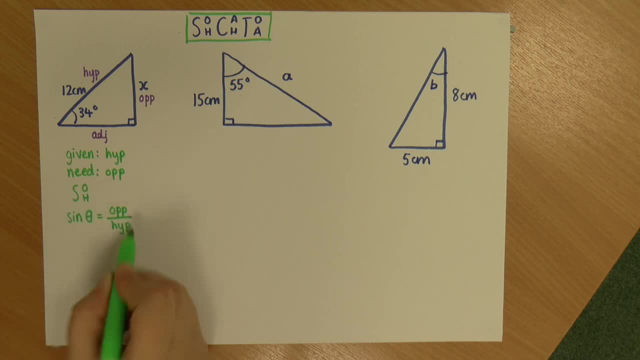 we've got our sine angle is equal to the opposite divided by the hypotenuse. So I'm going to start filling in these values. So my angle is 34 degrees. I always use that angle, I don't use the right angle. So sine 34 is equal to the opposite, which we don't. 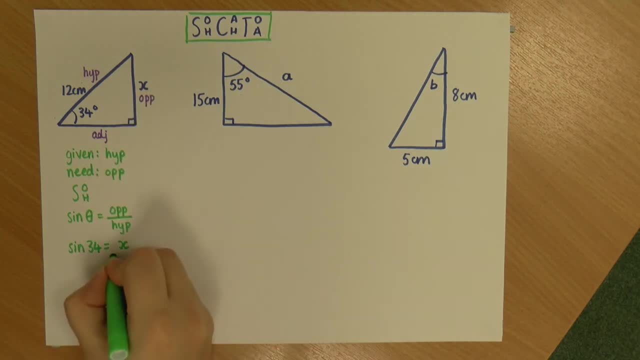 know. so I'm just going to put that in as x over the length of the hypotenuse, which is 12.. Okay, So now I need to rearrange this equation to give me x on its own, So I need to times both sides by 12.. 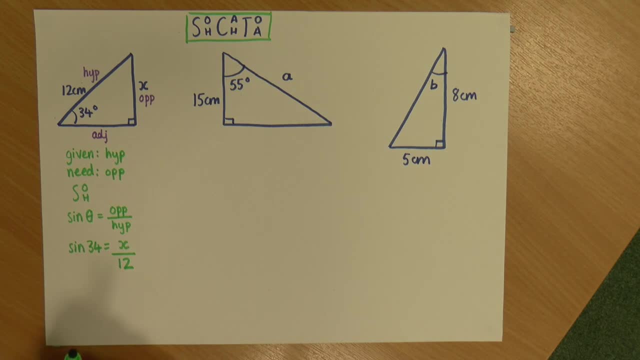 And if you're not sure what you're doing here, go and have a look at my videos on rearranging equations. But because we've got a division here, we are multiplying both sides by 12. We're doing the opposite. So that gives me sine 34 times 12 is x. 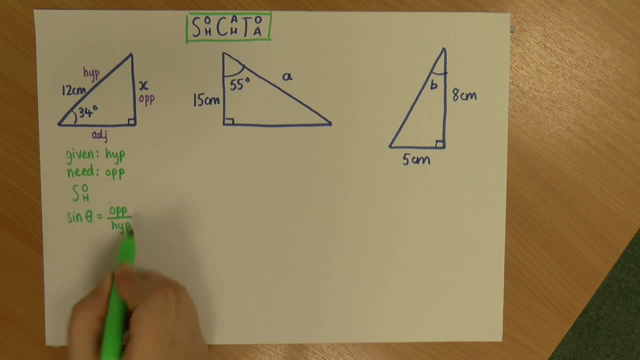 we've got our sign. angle is equal to the opposite divided by the hypotenuse. So I'm going to start filling in these values. So my angle is 34 degrees. I always use that angle, I don't use the right angle. So sign 34 is equal to the opposite, which we don't. 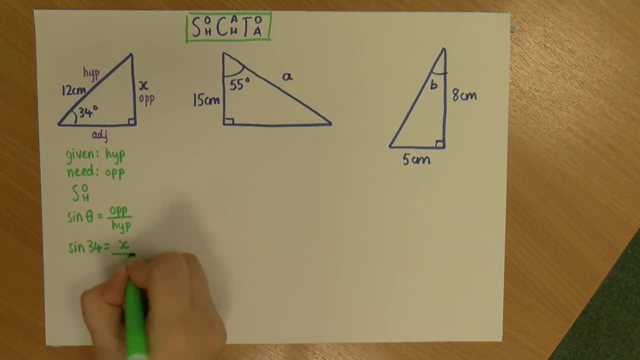 know. so I'm just going to put that in as x over the length of the hypotenuse, which is 12.. Okay, So now I need to rearrange this equation to give me x on its own. So I need to times. 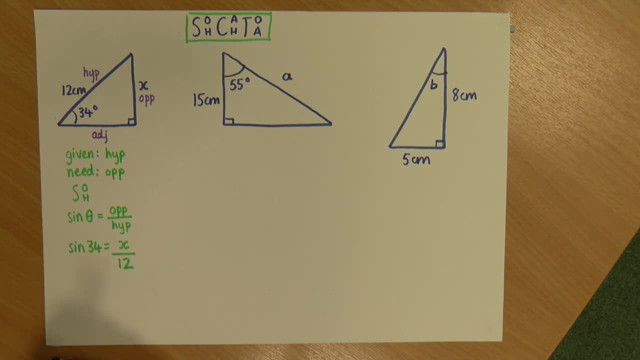 both sides by 12.. And if you're not sure what you're doing here, go and have a look at my videos on rearranging equations. But because we've got a division here, we are multiplying both sides by 12, we're doing the opposite. So that gives me sign 34 times 12 is x. So 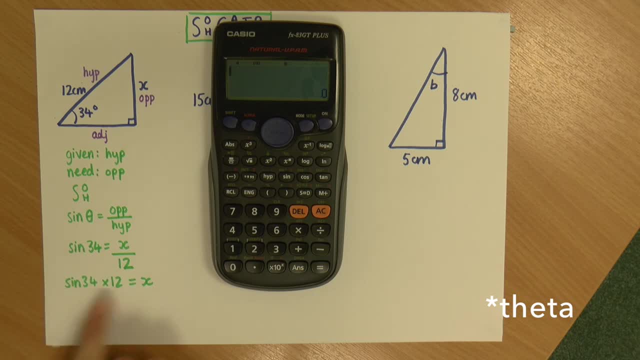 you will need a calculator for these. So I'm going to do sign 34,, sign 34, and I can press equals if I like: times 12.. There we go. So sign 34 times 12 gives me x, and x is 6.71, and my units are centimetres, because 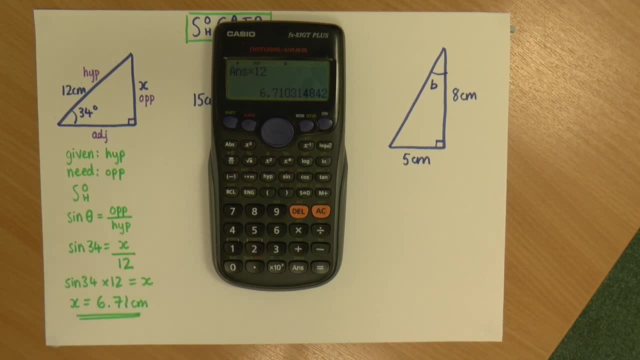 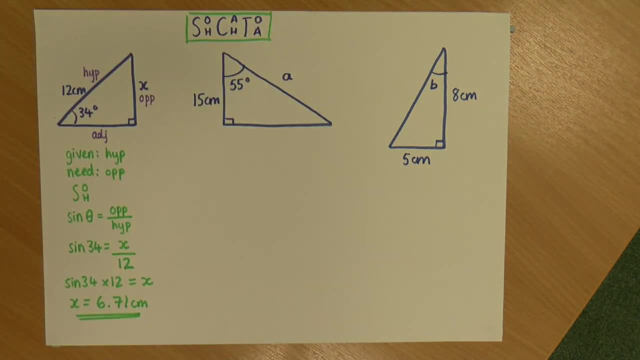 it's just the length of the side. Lovely, So that's it, Thank you. So that's the first one done where we've found the length of the opposite. Now for the middle triangle. So, again, the first thing I'm going to do is identify my 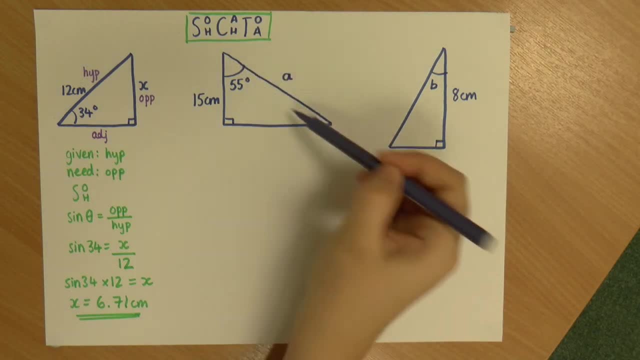 hypotenuse: opposite and adjacent. So my hypotenuse is the long diagonal opposite the right angle. So this is my hypotenuse. My angle is here, so my opposite is the side opposite it, which is this one, And my adjacent is the side next to it, which is this one. 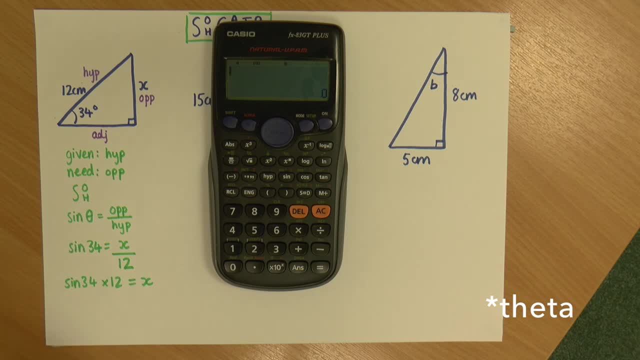 So you will need a calculator for these. So I'm going to do sine 34.. Sine 34. And I can press equals if I like, Times 12.. There we go. So sine 34 times 12 gives me x. 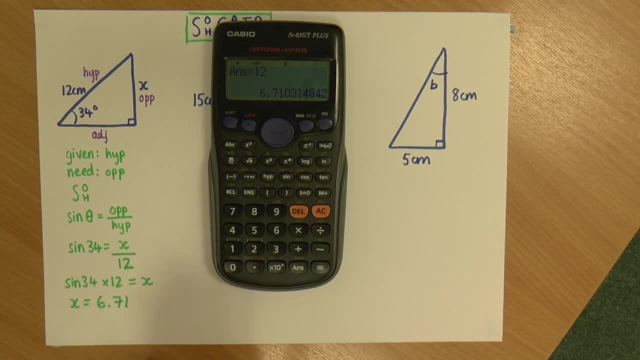 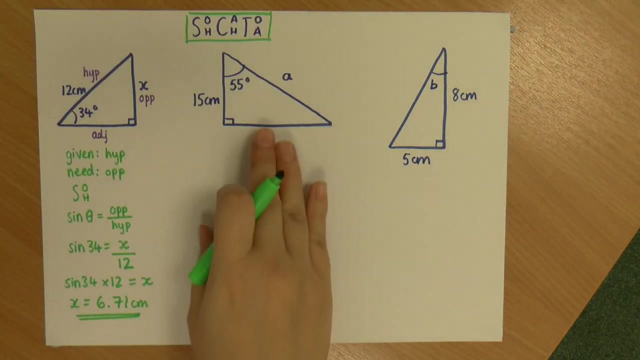 And x is 6.71.. And my units are centimetres, because it's just the length of the side, So Lovely. So that's the first one done, where we found the length of the opposite. Now for the middle triangle. So again, the first thing I'm going to do is identify my hypotenuse opposite and adjacent. 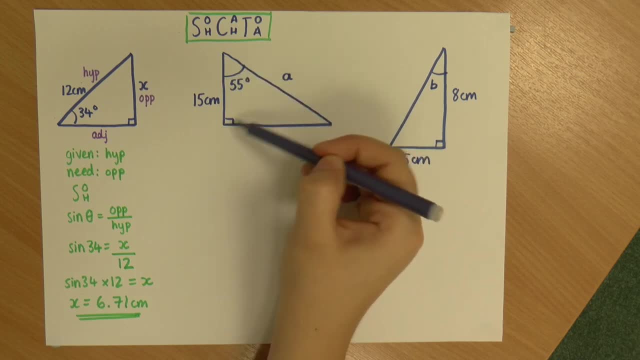 So my hypotenuse is the long diagonal opposite the right angle. So this is my hypotenuse. My angle is here. So my opposite is the side opposite it, Which is this one, And my adjacent is the side next to it, which is this one. 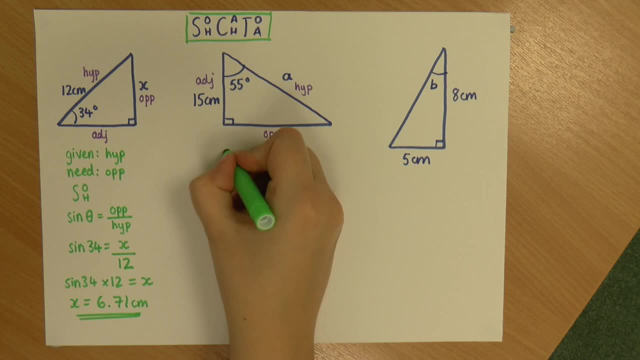 So again, let's see what we've been given and what we need. So we have been given this side, which is the adjacent, And we need side A, which is the hypotenuse. So A and H, We are looking which one of these contains the hypotenuse. 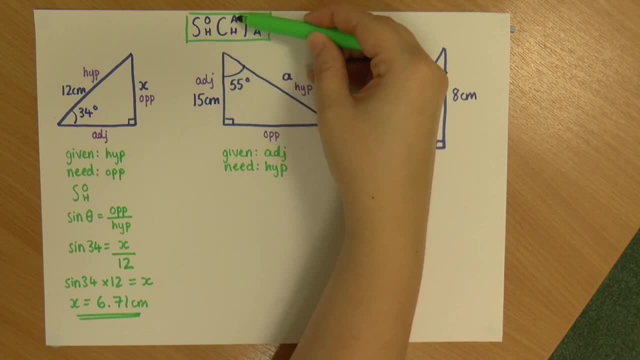 So it's the middle one, cos Cos contains A and H in its formula. None of the other do, So it's the one that looks like that, Or you may see it like that, And again I've used an x, this time instead of a sigma. 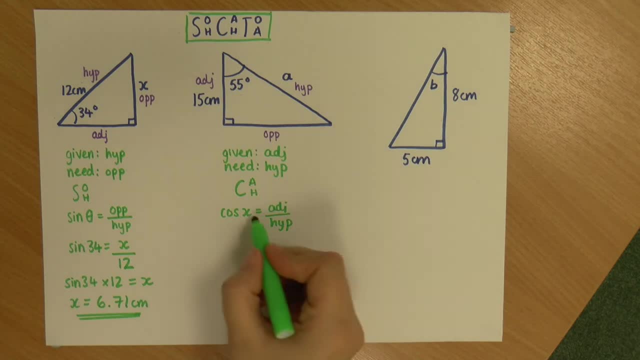 So this may look more familiar to you with an x, But again, that x is just the angle. Alright, so again I'm going to input my numbers. So my angle is 55. So cos 55 is equal to the adjacent, which we know is 15.. 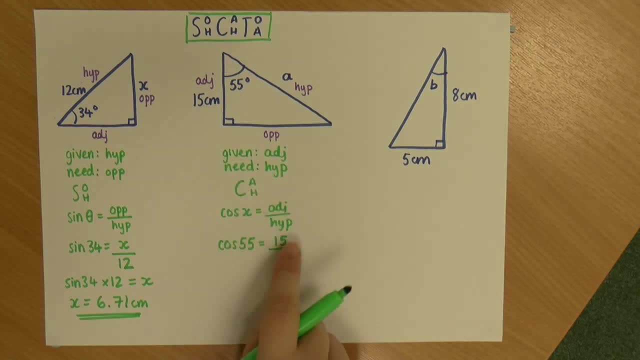 Divided by the hypotenuse, which is A. We don't know that yet, so I'm going to leave that as A. Now, with this one, we need to do a bit more rearranging, So the easiest way to find the hypotenuse: 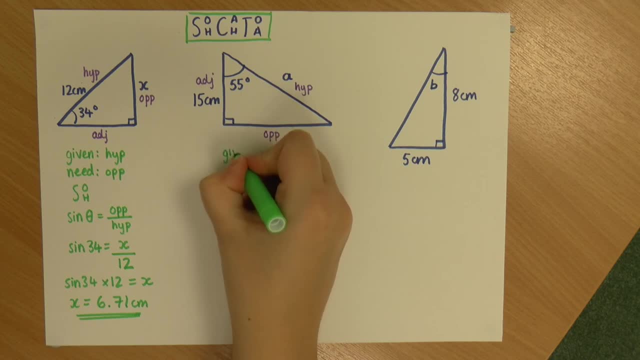 So again, let's see what we've been given and what we need. So we have been given this side, which is the adjacent, and we need side A, which is the hypotenuse. So A and H, we are looking which one of these contains them. 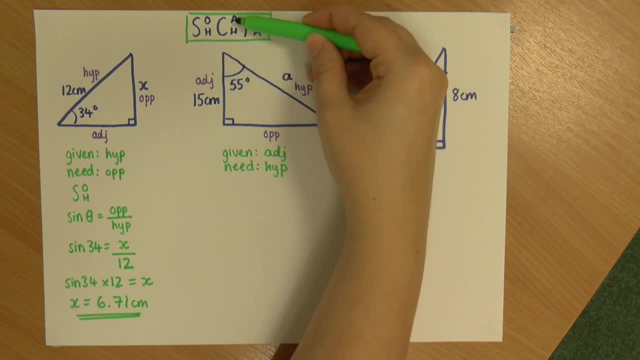 So it's the middle one, cos Cos contains A and H in its formula. None of the other do, So it's the one that looks like that, or you may see it like that, And again, I've used an X this time instead of a sigma, so this may look more familiar to you with an X. 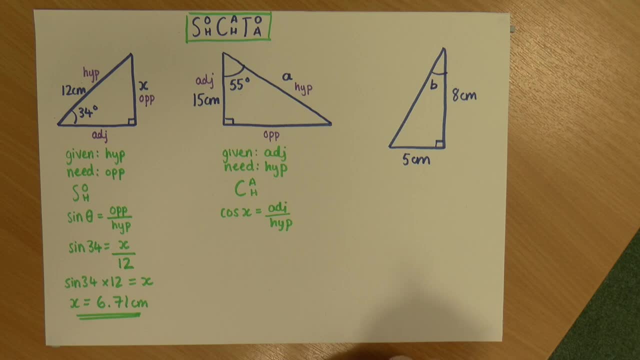 But again, that X is just the angle, All right. So again I'm going to input my numbers. So my angle is 55. So cos 55 is equal to the adjacent, which we know is 15, divided by the hypotenuse, which is A. 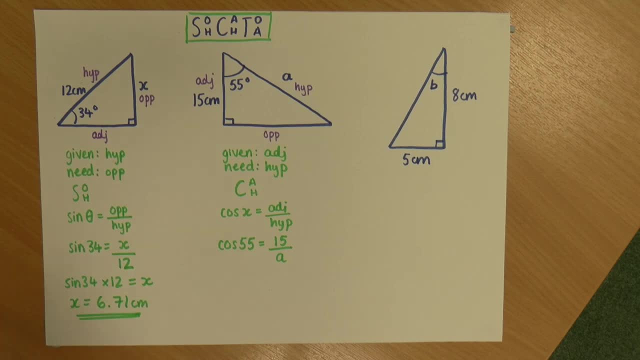 We don't know that yet, so I'm going to leave that as A Okay. Now, with this one, we need to do a bit more rearranging, So the easiest way to think about these things is to think about the hypotenuse. 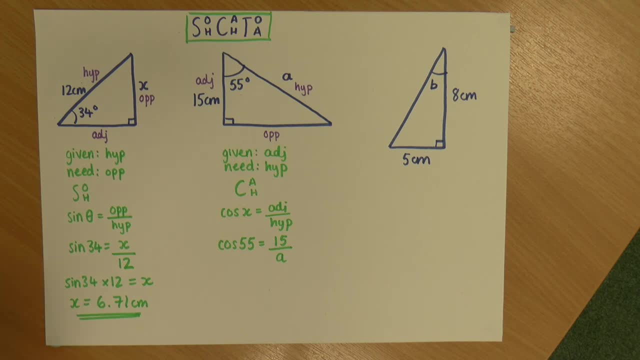 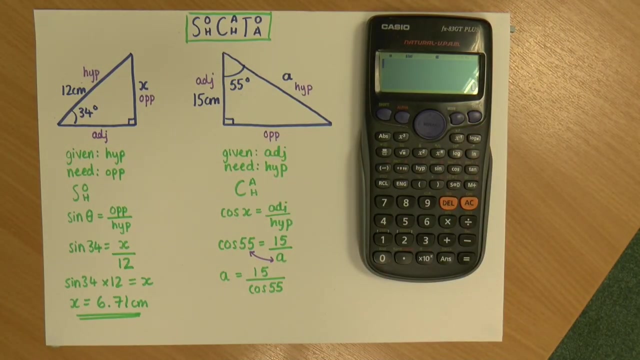 The easiest way to think about these types of formulae is to swap what's on the left of the equals and what's on the bottom. So if I do that, that gives me A is 15 over cos 55.. Lovely, If I grab my calculator again. 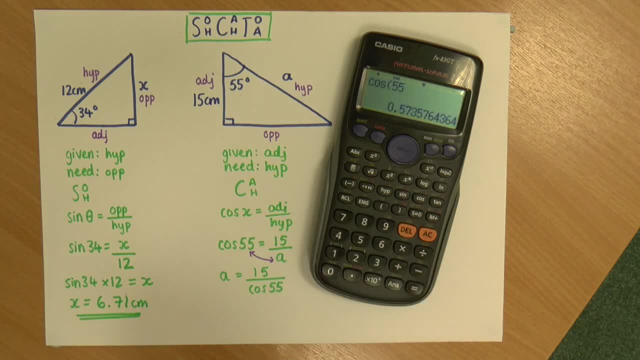 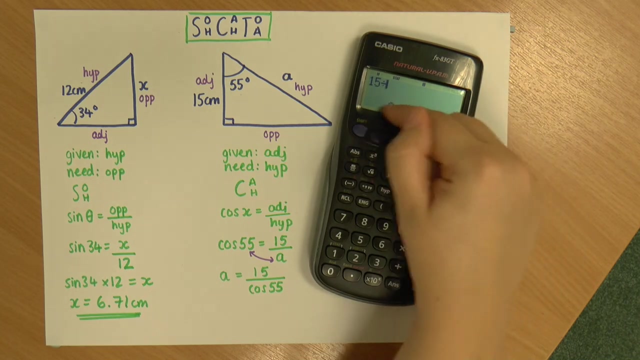 So this time I'm going to do cos 55. A is equal to that And I'm going to do 15 divided by it. So 15 divided by, And I'm going to use this answer button. So using that tells the calculator when I press it that the number I want to use is what is currently on the screen, what it's just done. 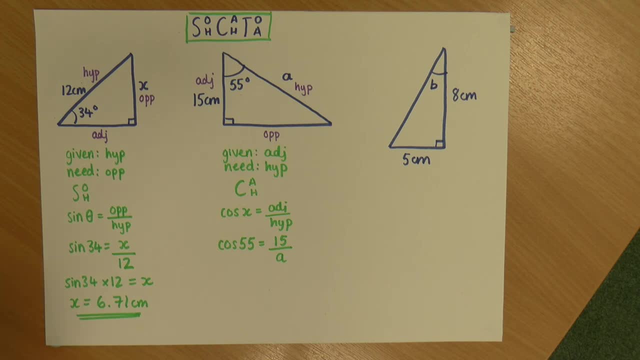 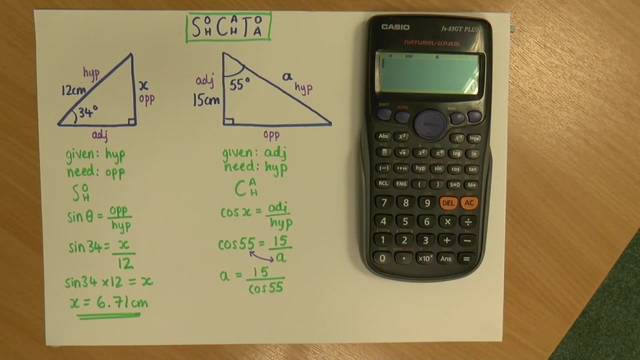 to think about these types of formulae is to swap what's on the left of the equals and what's on the bottom. So if I do that, that gives me A is 15 over cos 55.. Lovely, If I grab my calculator again. 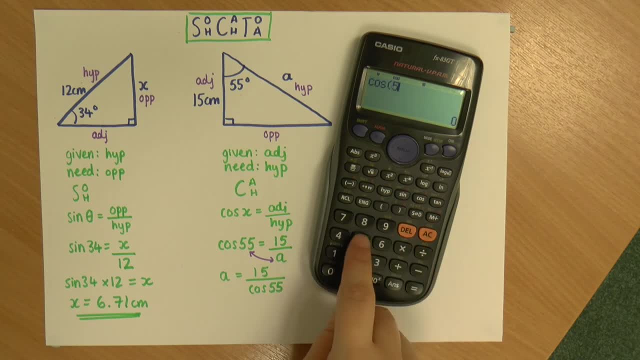 So this time I'm going to do cos 55. A is equal to that And I'm going to do 15 divided by it. So 15 divided by, And I'm going to use this answer button. So using that tells the calculator when I press it. 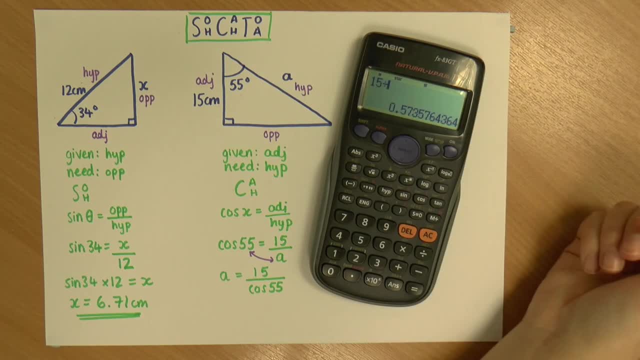 that the number I want to use is what is currently on the screen, what it's just done. So it's that cos 55.. So 15 divided by answer, And that gives me A, is equal to 26.2.. And again, it's a length, so it's centimetres. 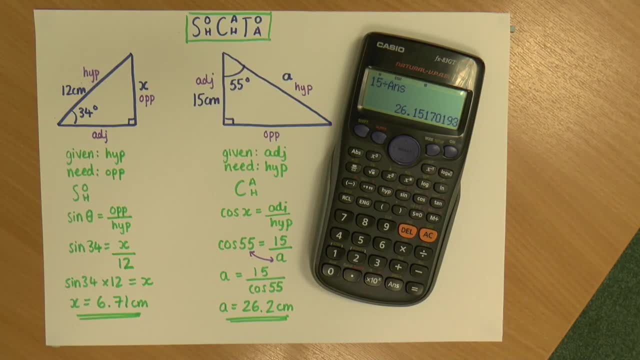 So that means my hypotenuse is 26.2.. And you can sort of check it common sense-wise because you'll know the hypotenuse is the longest side And this is longer than all the other sides we've been given. Well, the one side we've been given 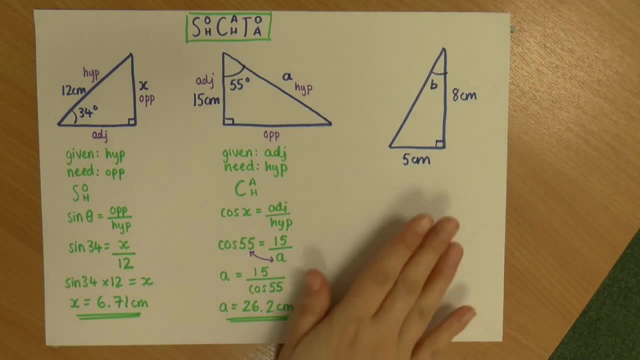 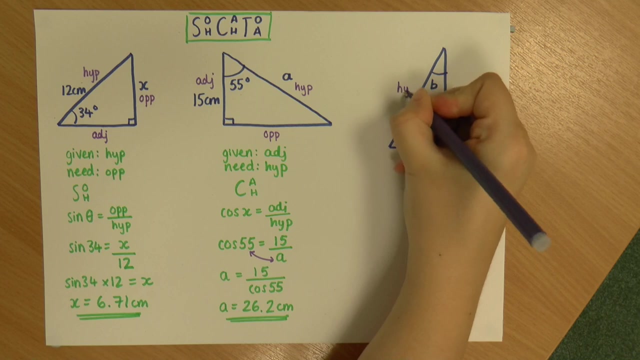 Perfect. Okay, And finally this last one. Now, this is a bit different. This is where we're finding a missing angle, not a missing side, But I'm still going to identify my three sides, So I've got my hypotenuse here. 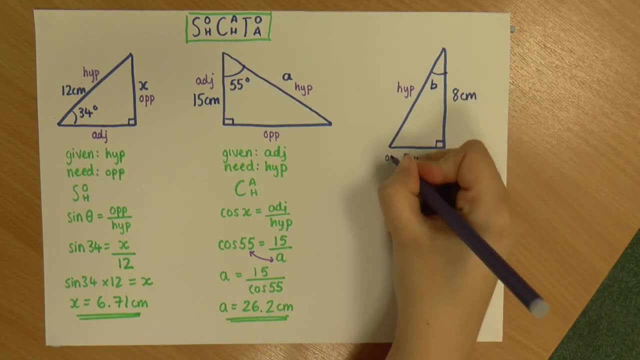 I've got my opposite down here And my adjacent on the right. Okay, So this time I have been given two sides. So I've been given this side, The opposite And the adjacent, And I'm being asked to find angle B. 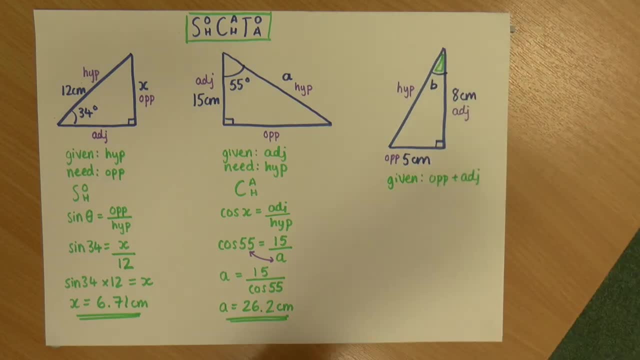 That's this one here, That angle there. So Which of the trigonometric functions uses the opposite and adjacent? Well, it's this last one. Opposite adjacent, It's tan Toa, Or again, you may see it written: 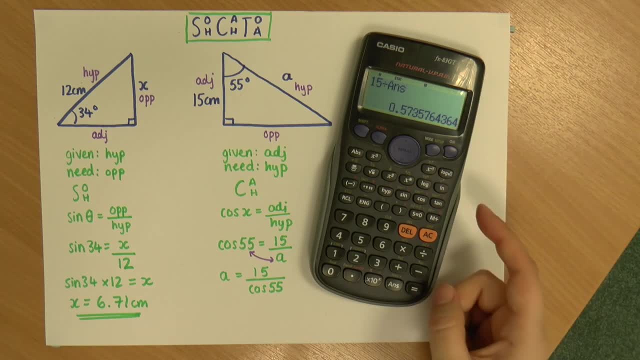 So it's that cos 55.. So 15 divided by answer, And that gives me A, is equal to 26.2.. And again, it's a length, so it's centimetres. So that means my hypotenuse is 26.2.. 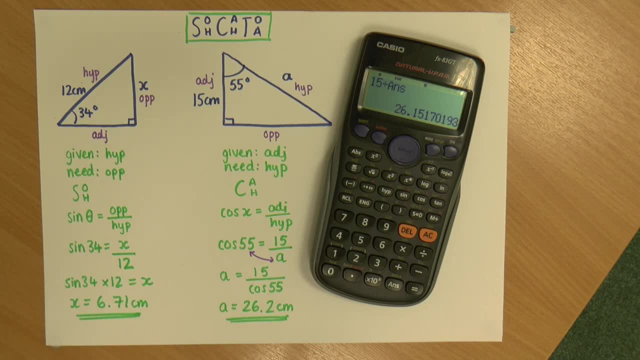 And you can sort of check it common sense-wise, because you'll know, the hypotenuse is the longest side And this is longer than all the other sides we've been given. Well, the one side we've been given, Perfect, Okay. 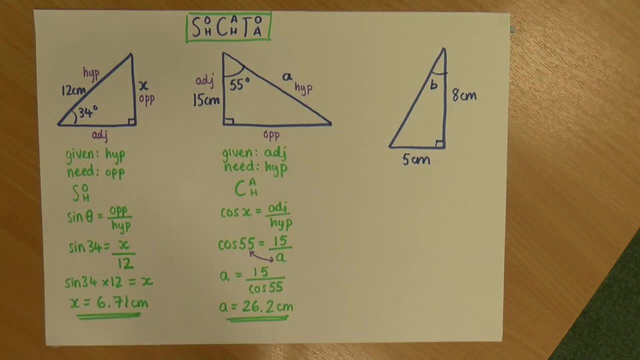 And finally this last one. Now, this is a bit different. This is where we're finding a missing angle, not a missing side, But I'm still going to identify my three sides, So I've got my hypotenuse here. 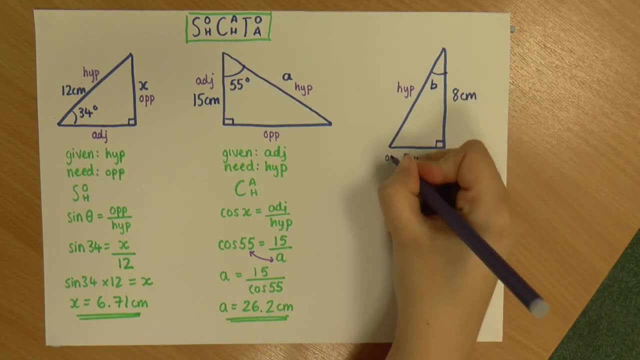 I've got my opposite down here And my adjacent on the right. Okay, So this time I have been given two sides. So I've been given this- The opposite And the adjacent, And I'm being asked to find angle B. 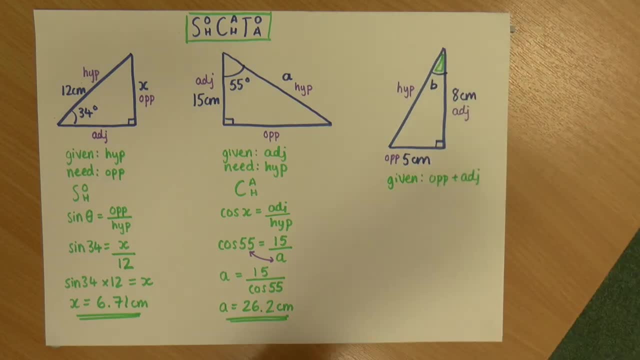 That's this one here, That angle there. So Which of the trigonometric functions uses the opposite and adjacent? Well, it's this last one. Opposite adjacent, It's tan Tauor, Or again, you may see it written: 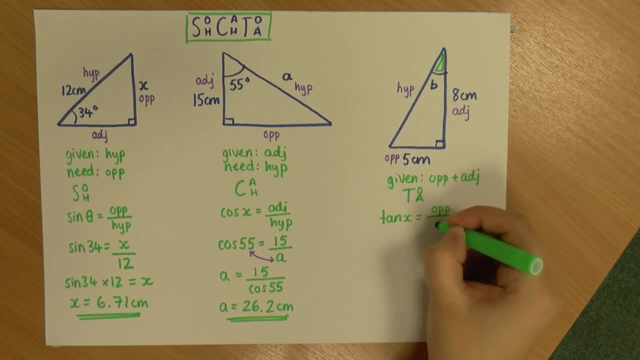 Tan x is opposite over adjacent. Okay, So, like with the others, I'm going to start off by popping some numbers in. So this time my angle is just B, I don't know it yet. My opposite is 5.. 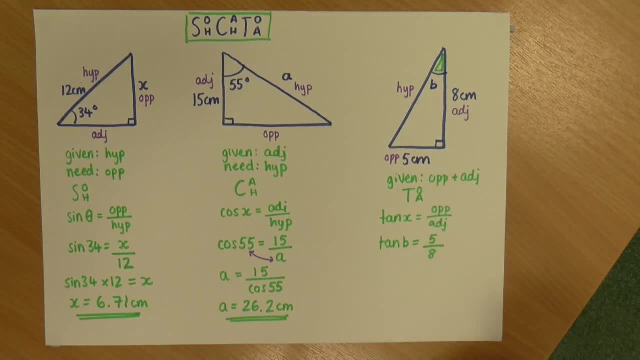 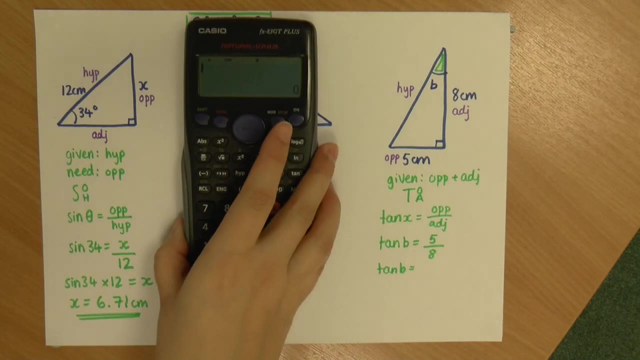 And my adjacent is 8.. Okay, So tan B And I'm going to do 5 divided by 8. And I'm actually going to pop it in a calculator: 5 divided by 8. And that gives me 0.625..